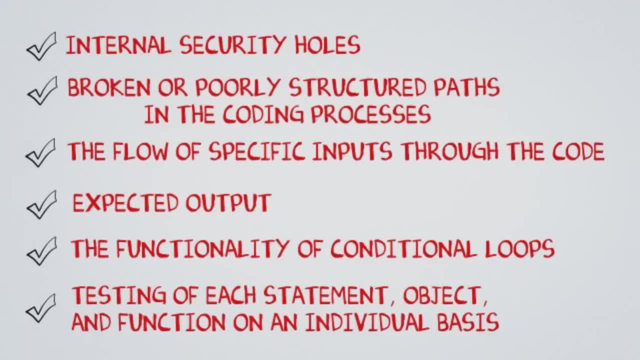 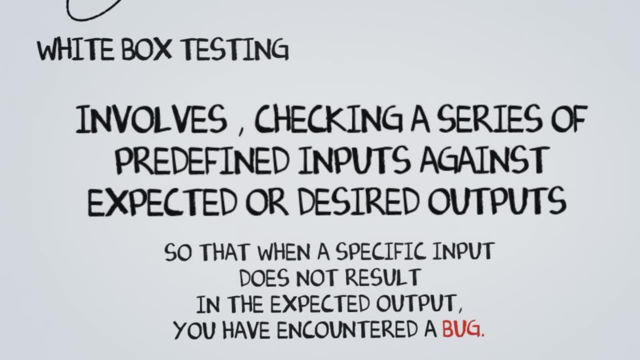 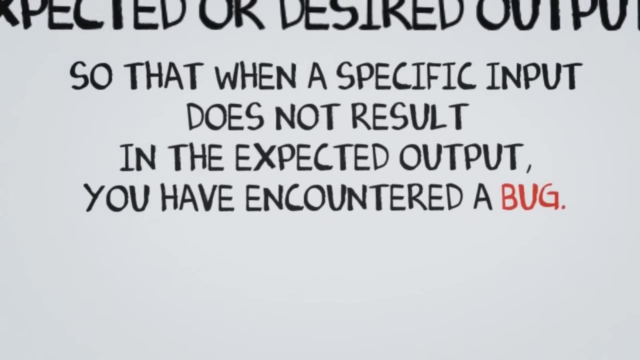 loops and testing of each statement, object and function on an individual basis. White box testing involves checking a series of predefined inputs against expected or desired outputs, so that, when a specific input does not result in the expected output, you have encountered a bug. How do you perform white box testing? To give you a simplified 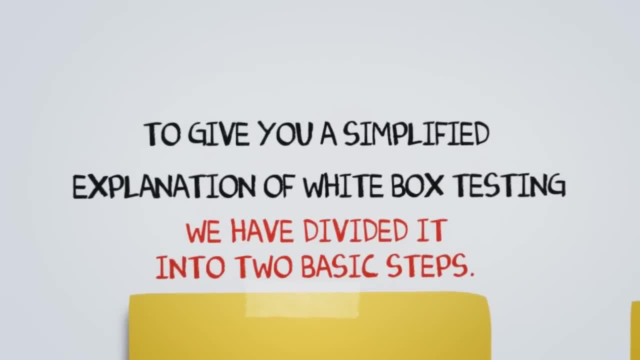 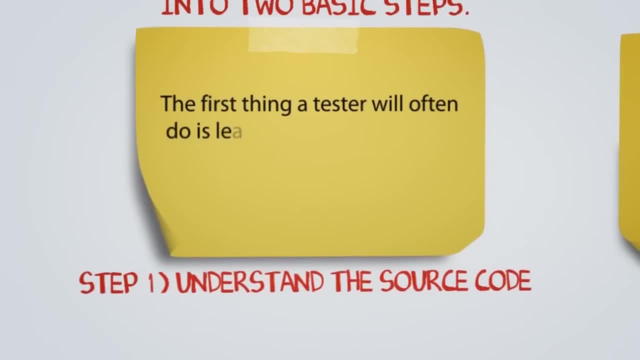 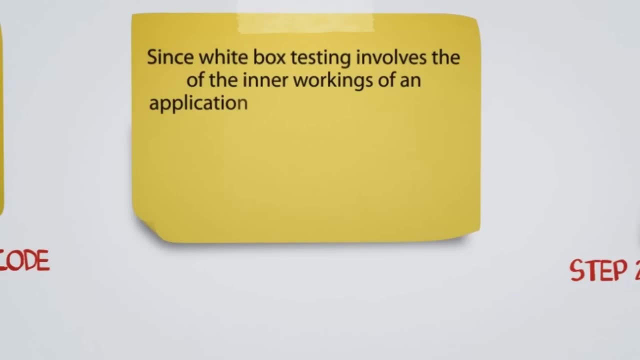 explanation of white box testing. we have divided it into two basic steps. Step one: understand the source code. The first thing a tester will do is learn and understand the source code of the application, Since white box testing involves the testing of the inner workings. 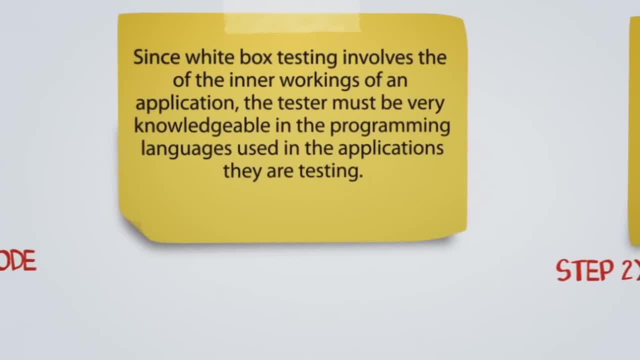 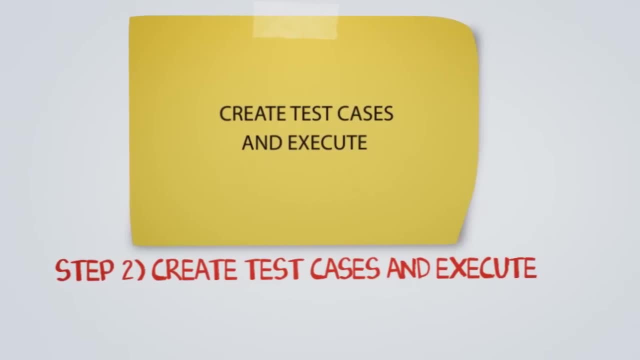 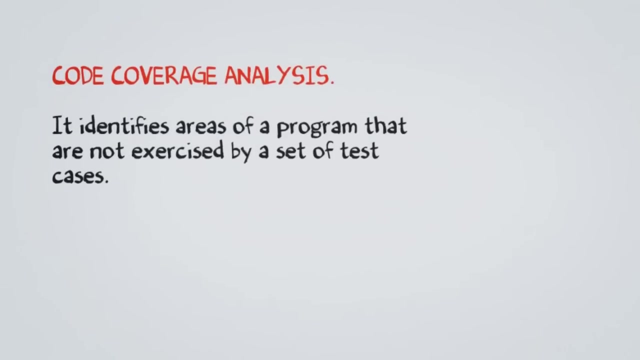 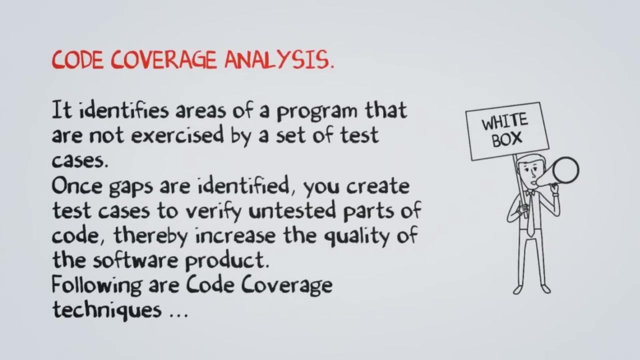 of an application. the tester must be very knowledgeable in the programming languages used in the applications they are testing. Step two: create test cases and execute White box testing techniques. Code coverage analysis: It defines areas of a program that are not exercised by a set of test cases. Once gaps are identified, you create test cases to. 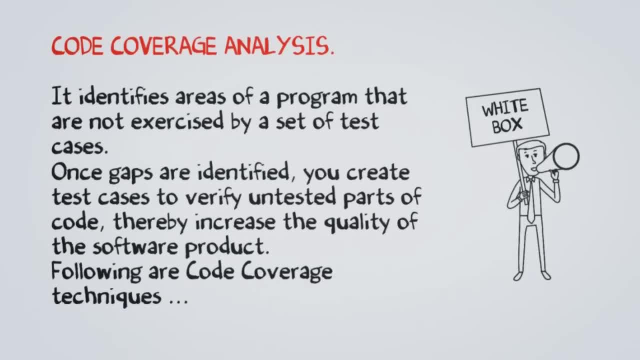 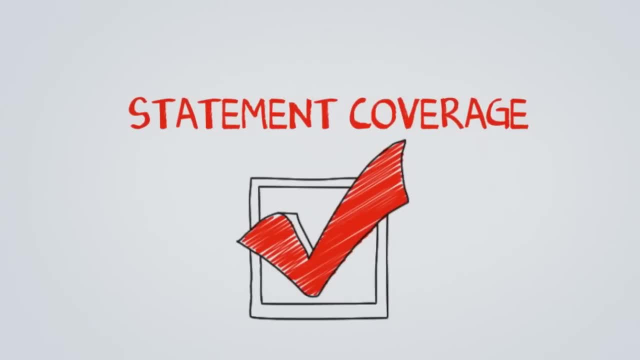 verify untested parts of code, thereby increasing the quality of the software product. Following our code coverage techniques, you will be able to verify the quality of the software product, making sure you have a clear understanding of the code. Setting the code for testing gives a. 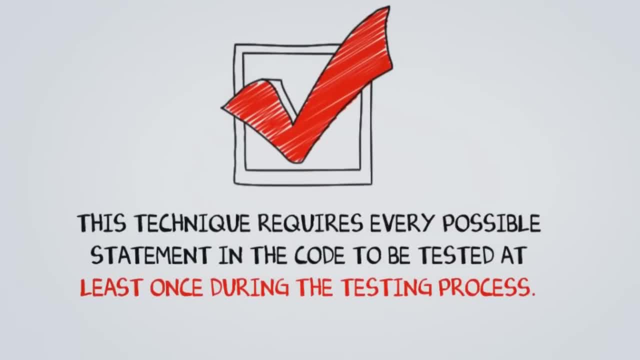 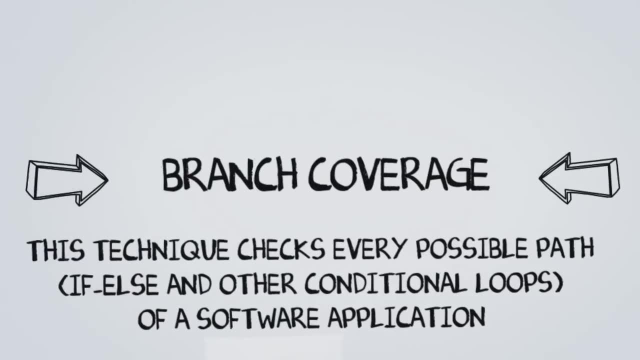 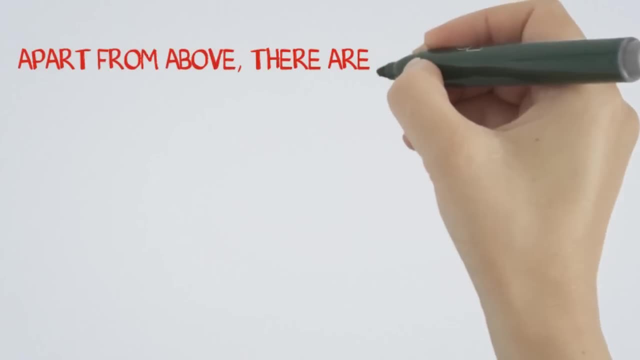 more precise understanding of the code. This technique requires every possible statement in the code to be tested at least once during the testing process. Brace coverage: This technique checks every possible path of a software application. Apart from above, there are numerous coverage types, such as condition coverage. 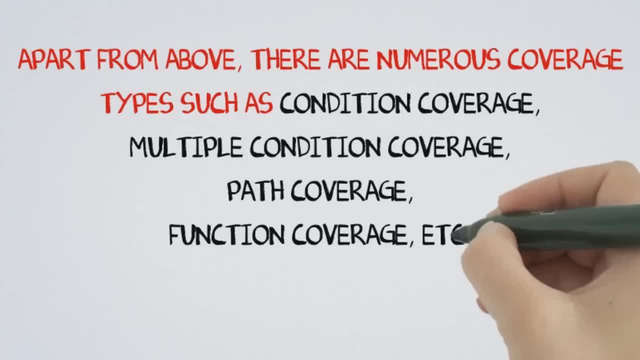 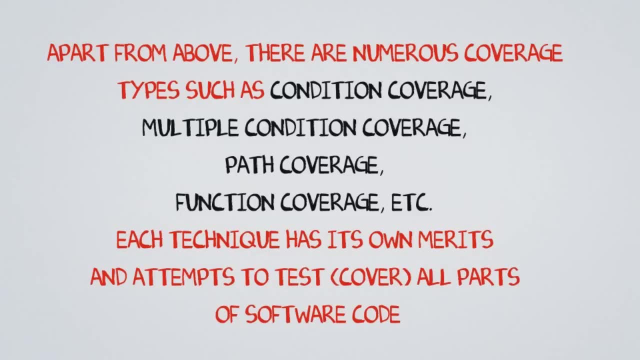 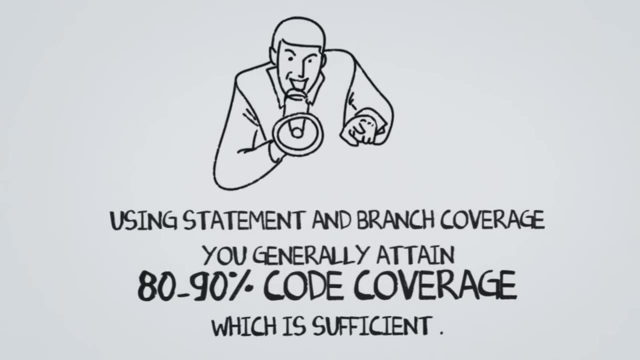 multiple condition coverage, path coverage, function coverage coverage, etc. Each technique has its own merits and attempts to test or cover all parts of the software code. Using statement and branch coverage, you generally attain 80-90% code coverage, which is sufficient. 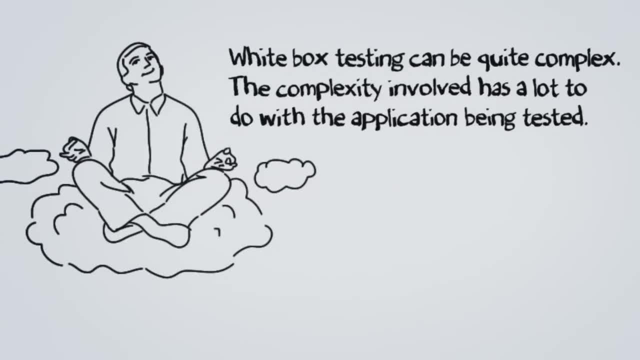 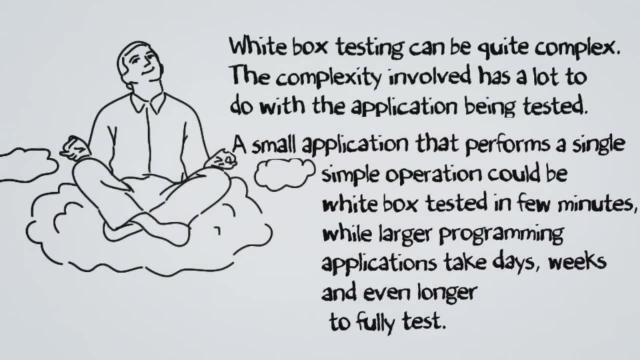 Conclusion: White box testing can be quite complex. The complexity involved has a lot to do with the application being tested. A small application that performs a single simple operation could be white box tested in a few minutes, with larger programming applications taking days, weeks or even longer to fully test.